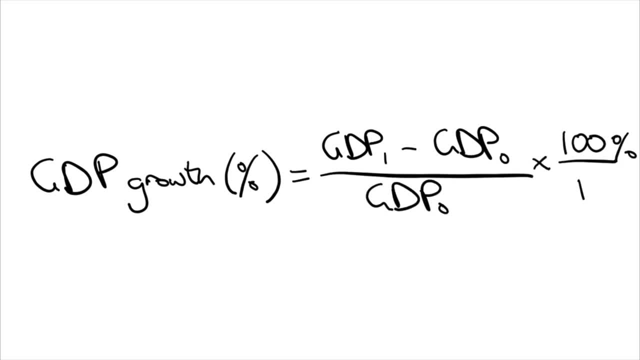 last year, expressed as a percentage of last year's growth. Positive economic growth is important because it means that we are producing more goods and services to satisfy wants and needs, And in doing so, we are also earning more income. Why does economic growth fluctuate, though? 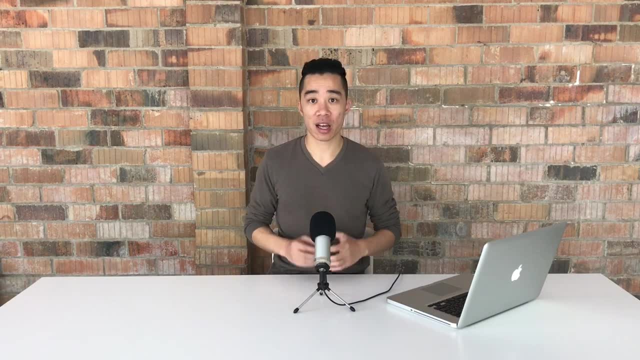 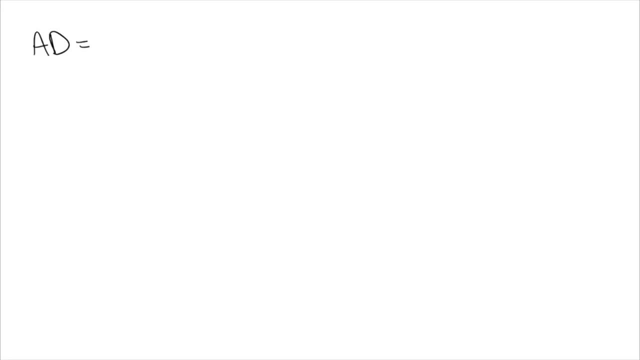 One explanation that we learned in the HSC course is aggregate demand. Aggregate demand is the sum of all expenditure on domestic output in the economy. This is broken down and calculated by adding up consumer spending by households, investments by firms, expenditure by governments. 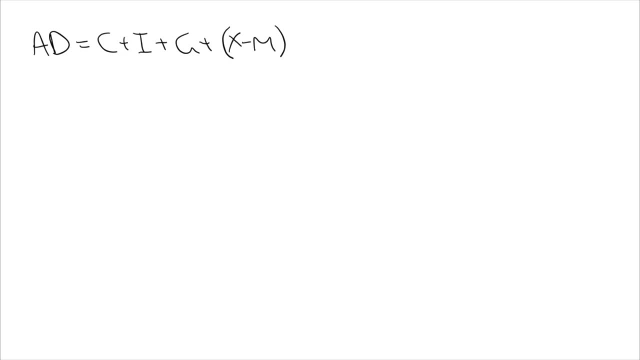 and net exports, which is exports minus imports. So what's this got to do with economic activity? Well, an increase in aggregate demand leads to increased expenditure, which reflects higher output and income. You can see this in this aggregate demand diagram too, And a decrease 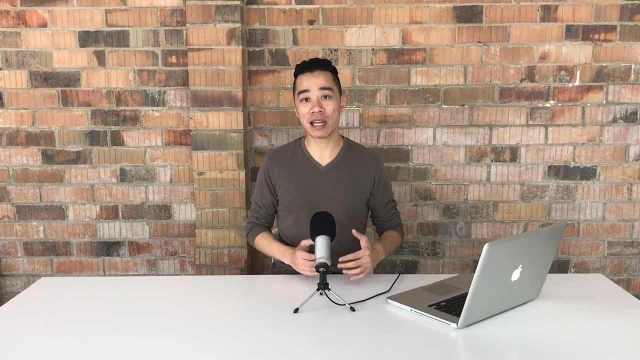 in aggregate demand will cause a downswing instead. That's why I believe this formula is arguably the most important formula in the whole course. Almost every short-term movement in economic growth is explained by the components in this formula. For example, what caused our GDP growth? 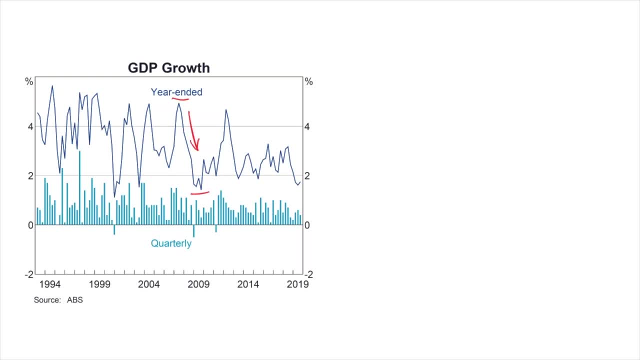 rate to fall from 4.3% in 2008 to a low of 1.8% in 2009?. It was the global financial crisis, or GFC, which started from the US housing crisis. It caused trade and foreign investment to decrease. 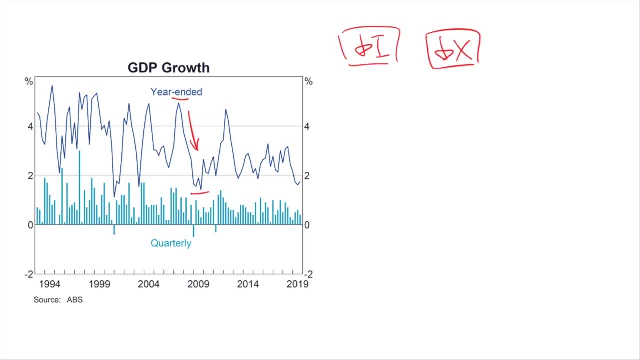 around the world, meaning less investment and net exports into Australia. Furthermore, consumer confidence and investor confidence also fell further, lowering aggregate demand and economic activity, And that's why I believe this formula is important, And that's why I believe this formula is important, And that's why I believe this formula is important. And then, what caused the? 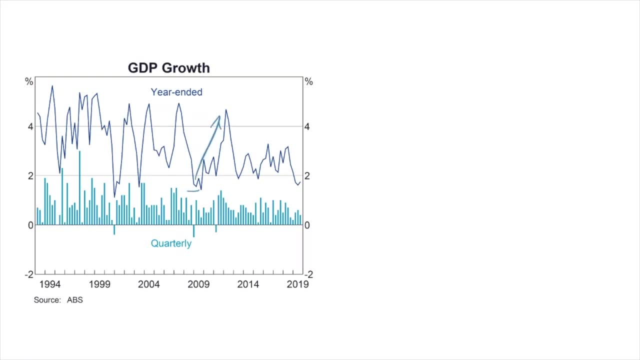 second mining boom, where GDP growth went from 1.8% in 2009 to a peak of 3.9% in 2012?. Kevin Rudd's government expenditure in 2009 helped to kickstart economic activity. More importantly, China's. 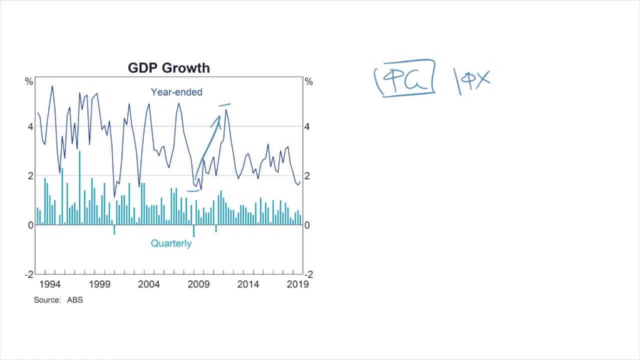 economy was increasing production, causing demand for Australian exports to increase. China also contributed high levels of foreign investment into Australia. Australian consumer and investor confidence subsequently increased, contributing to an increase in aggregate demand and an economic boom. The subsequent increase in GDP growth led to a rise in GDP growth. And then what caused the? 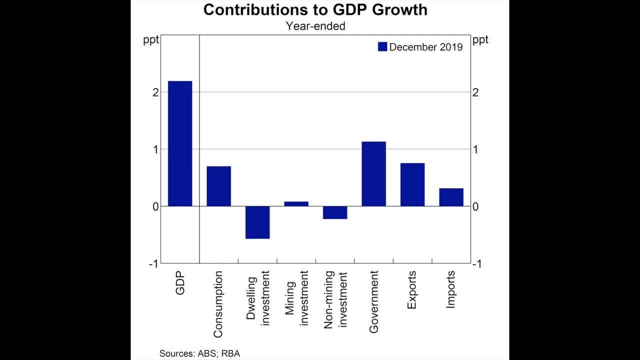 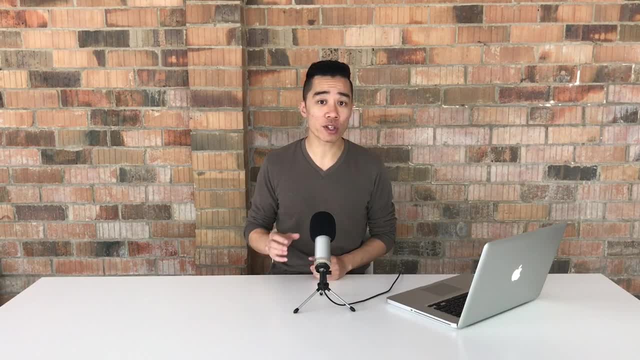 certificate of equitable and rationalciąg on trade WILLIAM. The subsequent movein cts in economic activity can also be explained by movements in the components of aggregate demand. At the time of recording this video, we're in social isolation due to the coronavirus. We haven't gotten all of the economic figures yet. But which components of aggregate demand do you think are affected? What are the flawed effects on other economic issues? What are the RBA, state governments and federal governments doing to influence aggregate demand? Get into a habit of noticing these concepts in the spirit of real life. L paws in the ficou. life. Gum banana for Não, because it could help solidify your understanding Again. leave it out there and enjoy the rest of the research. We take a, друзья, The top ten Hyundai cerealeler. Go to the at home alone net supermarket. You want an? 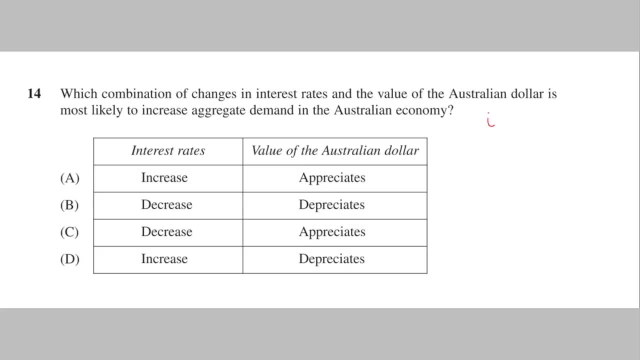 practice what we've learned today with some HSC questions. In 2013's HSC question 14,, we're asked which of the following scenarios will increase aggregate demand. Firstly, a decrease in interest rates would cause an increase in consumption, as existing borrowers of debt would have more. 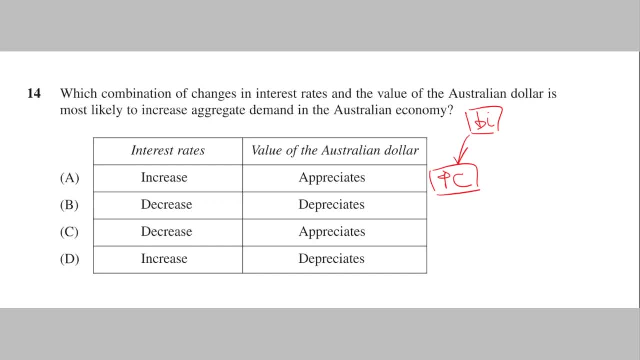 disposable income. They would also have less reward for saving. Investors could also find it easier to borrow to invest. This all leads to increased aggregate demand, which is why the RBA lowers cash rates to stimulate economic growth. This will be covered in more detail when we look. 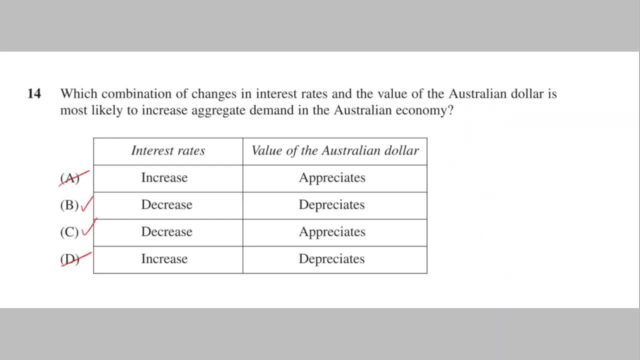 at economic policies. Anyway, we know the answer is either B or C. If the Aussie dollar depreciates, Aussie exports look more affordable to foreign buyers so we can sell more, and foreign imports look more expensive to Australians, so we buy less. This means net exports will increase. 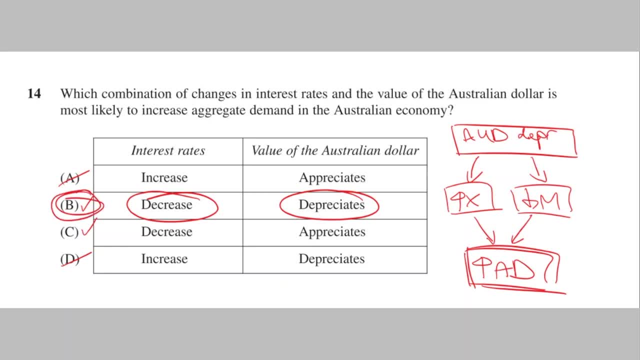 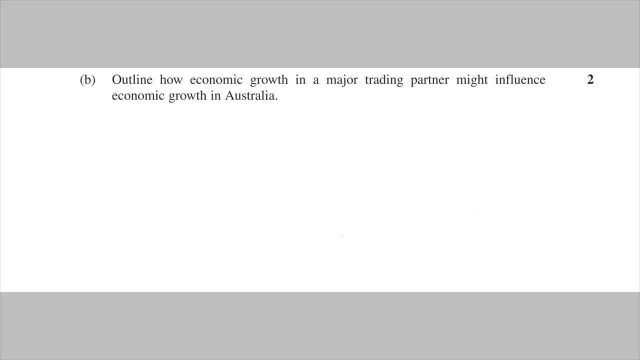 causing an increase in aggregate demand. The answer is therefore B, Also from the same year's HSC paper. we can have a go at a short answer question. It requires two marks worth of detail about how an increase in growth in a trading partner can influence economic growth. 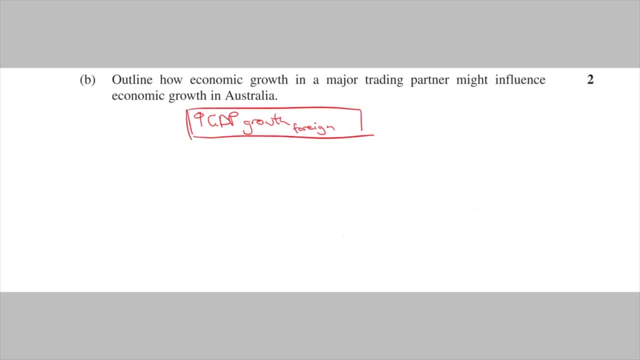 Well, if our trading partner is experiencing economic growth, they will have more disposable income and will be increasing production. This means that their demand for Australian products and imports will increase, causing an increase in net exports and, in turn, aggregate demand and economic growth in Australia. An alternative link that you could make is that with economic growth.